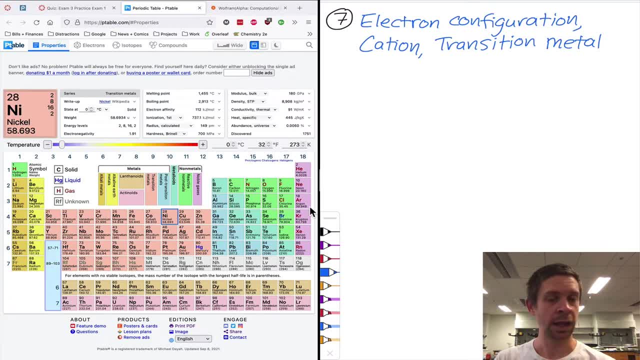 What row am I in? First of all, I'm in row 4. And I know that the core of a nickel atom includes all of the electrons up to argon, And so you know. to start things off, I can say that the electron configuration of nickel 2 plus 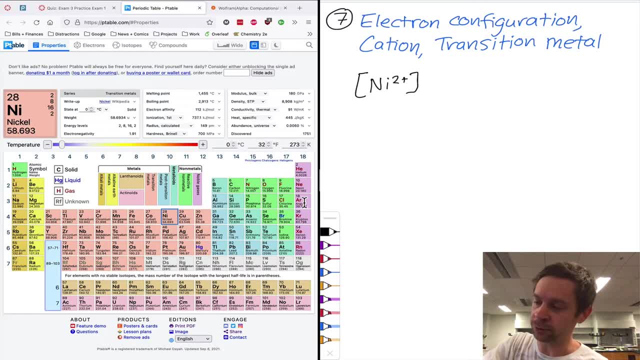 which hasn't lost any core electrons, which is normal for stable cation, is going to include all of the electrons of argon in their corresponding shells, subshells etc. and start there. I may also start by thinking about the electrons in the 4S subshell. 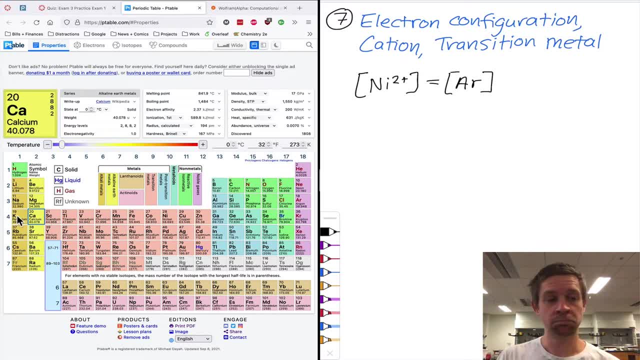 and thinking, for example, about 4S2, two electrons in the 4S subshell and 1,, 2,, 3,, 4,, 5,, 6,, 7, 8 electrons in the 3D subshell. 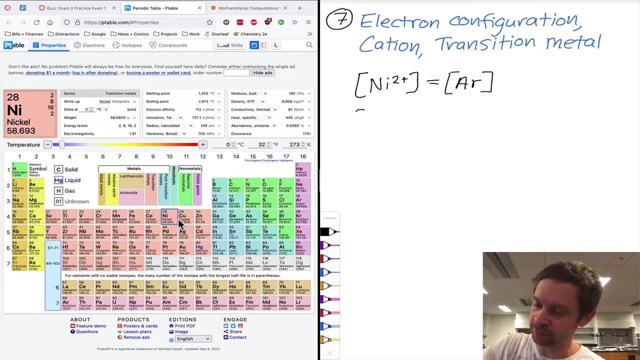 for a neutral nickel atom, and let's actually write that down separately. So for a neutral nickel atom we'd be looking at all of those electrons in argon. 4s23d8 would be the electron configuration of a neutral nickel atom. right, just naively proceeding. 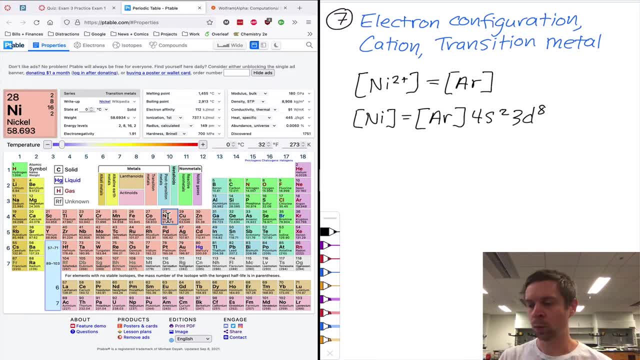 across the periodic table. Now what happens when a transition metal atom loses electrons? Remember that those energy levels jiggle, So a level that was higher in energy, the 3d subshell, can dip below the 4s subshell. 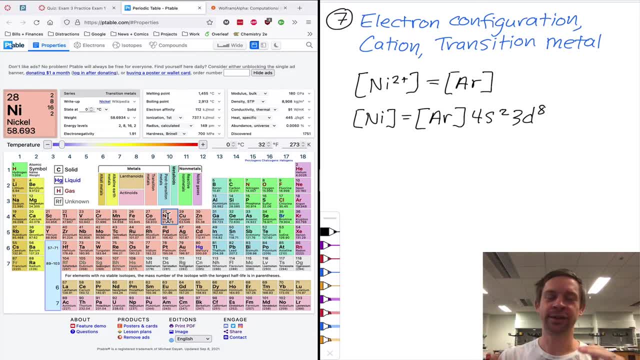 in energy, and that's exactly what happens for transition metal kaions. As soon as they lose an electron, the energy of the 3d subshell goes down quite a bit relative to 4s, And this has to do with the fact that the 3d orbitals, or electrons in the 3d orbitals, 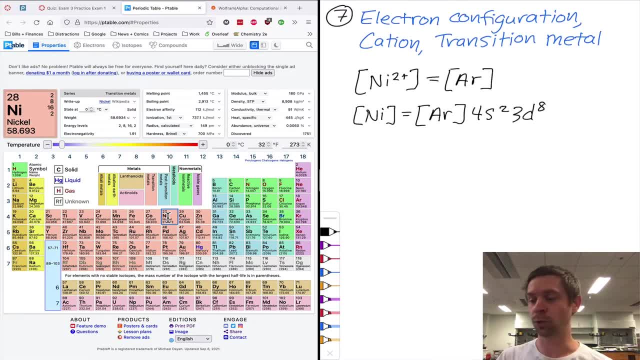 are actually, on average, closer to the nucleus than 4s electrons, And so as the effective nuclear charge of the valence shell goes up, those 3d electrons decrease in energy faster than the 4s electrons. So that's a long-winded way of saying that, in order to proceed in going from neutral. 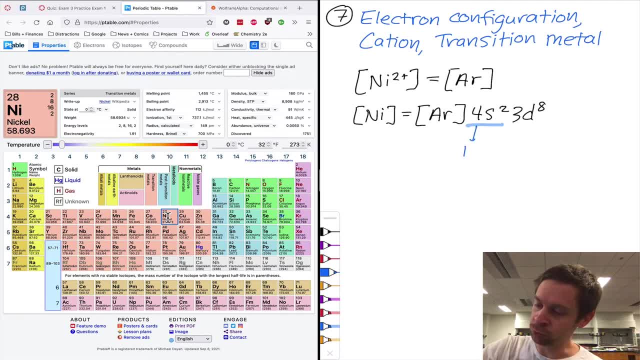 nickel to nickel 2+, we're going to lose both of those electrons. And we're going to lose two electrons because the charge of the ion we're interested in is nickel 2+, and both of those electrons come from the 4s subshell. 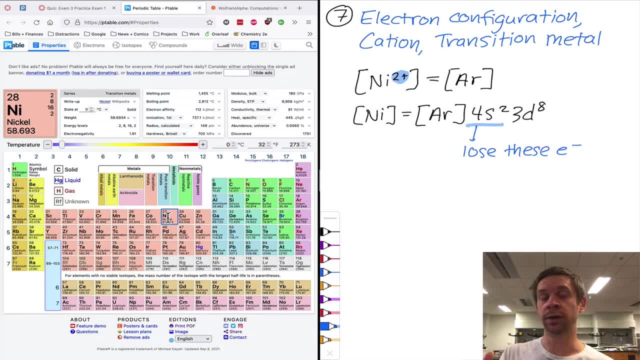 If we only lost one electron, actually the same idea would apply and we would take that remaining 4s electron and put it down down now, because the 3d level is below the 4s in energy- into a 3d orbital, leading to a 3d subshell. 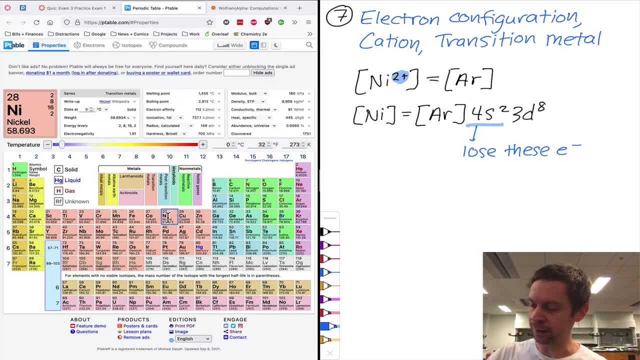 So that's a long-winded way of saying that, in order to proceed in going from neutral nickel to nickel 2+, we're going to lose both of those electrons, and in this case we're going to lose both of those electrons in the 4s subshell and go straight to a 3d8 situation. 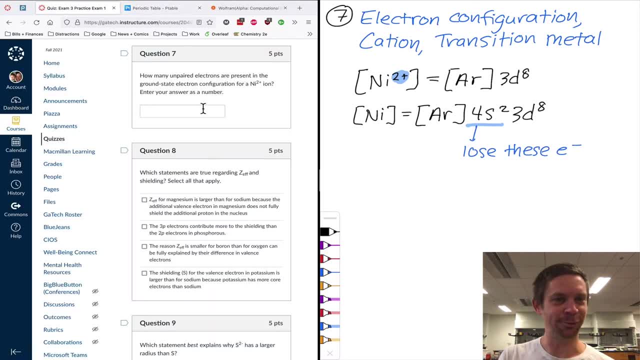 Now, in terms of actually answering the problem, how many unpaired electrons are present in the ground state electron configuration of a nickel 2+ ion? let's get an orbital energy diagram down to unpack this. So energy on the y-axis and actually to illustrate a point that I made earlier, just 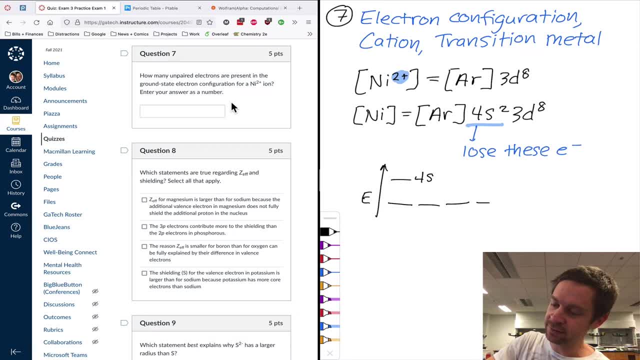 waving my hands around In the cation, the 3d subshell is lower in energy than the 4s subshell. I know I've got 8 valence electrons based on nickel 2+- based on the number of electrons in a nickel 2+ ion- and I'm just going to start filling the 3d subshell with those 8. 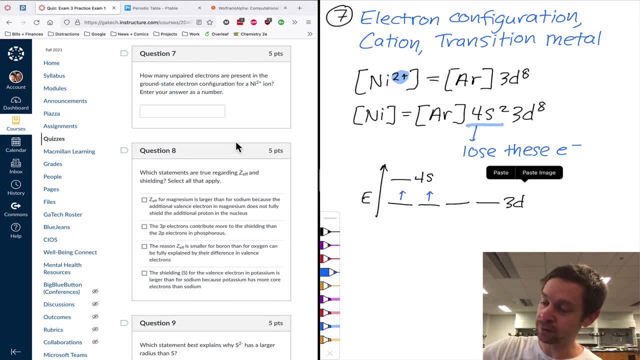 electrons in accordance with the Aufbau principle and Hund's rule. So 1,, 2,, 3,, 4,, 5,, 6,, 7., 8, and I'm realizing that I have missed an orbital in the 3d subshell. 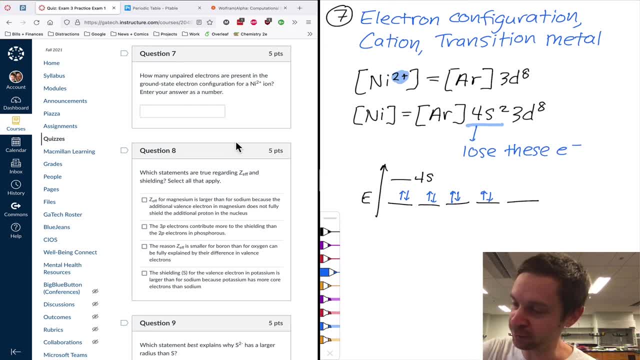 It's got 5,, not 4, and, if my math is serving me correctly, here we're going to need to take one of those electrons and put it there. You know what? Let's just start over, because I want to illustrate Hund's rule in action. 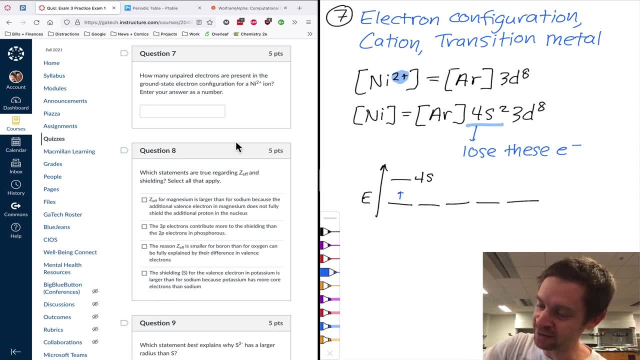 As you're filling electrons into d orbitals, the first 5 electrons will all go into unique orbitals within the 3d subshell, like so, And then, to finish this off, we're going to do 6,, 7,, 8,, pairing those last 3 electrons.